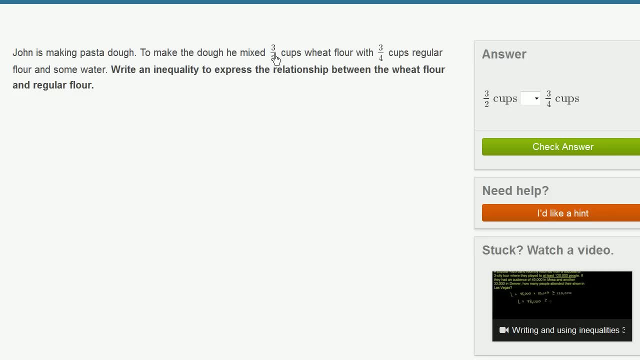 So he mixed 3 1⁄2 cups of wheat flour. 3 1⁄2 is the exact same thing as 1 and 1 1⁄2 if we were to write it as a mixed number. So it's more than 1 cup of wheat flour. 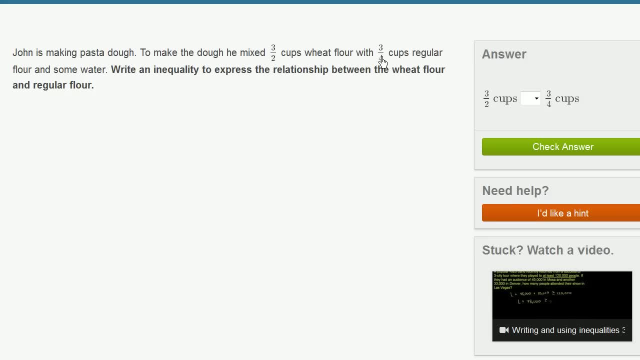 And he mixes that with 3 1⁄4 cups of regular flour. Well, 3 1⁄4 is less than 1.. So 3 1⁄2 is definitely greater than 3 1⁄4.. 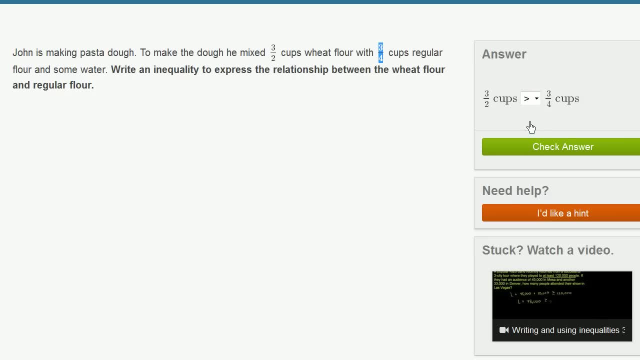 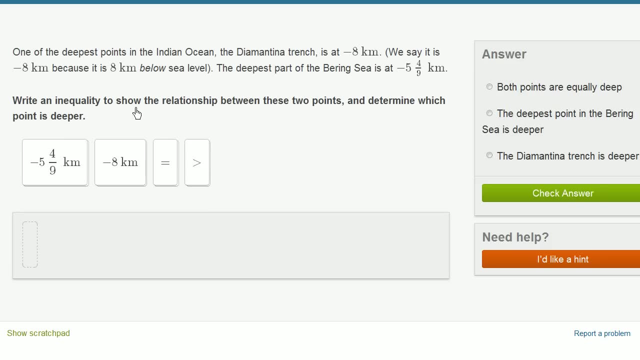 And we can write that We can just pick greater than right over there. 3 1⁄2 is greater than 3 1⁄4.. Let's do a couple more of these. One of the deepest points in the Indian Ocean. 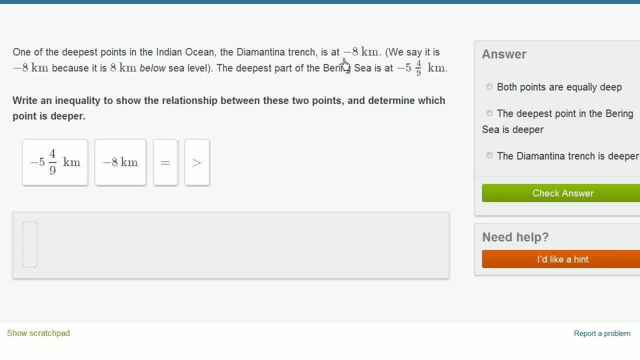 the Dimantina Trench is at negative 8 kilometers. We say it is negative 8 kilometers because it is 8 kilometers below sea level. The deepest part of the Bering Strait is at negative 5 and 4 1⁄9 kilometers. 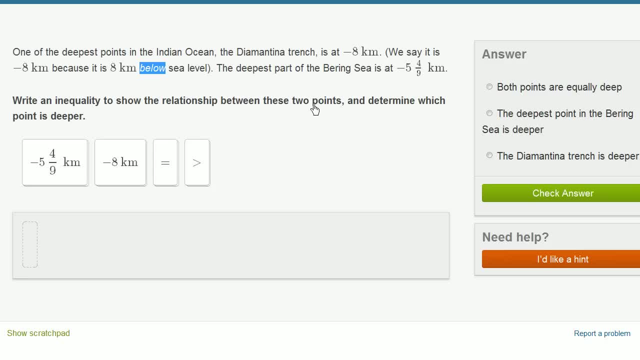 Write an inequality to show the relationship between these two points and determine which point is deeper. So let's say we have a greater than sign here, So we want to write whichever quantity is greater on the left-hand side. So we look right over here. 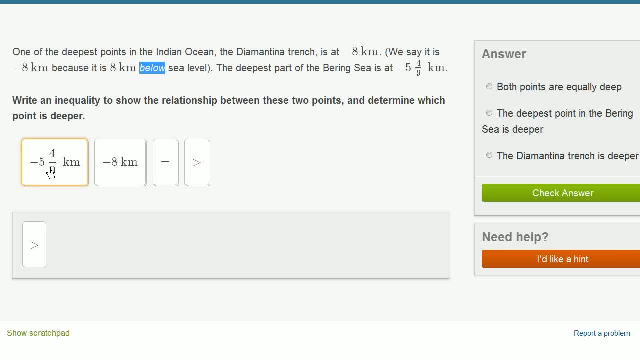 This number 5.. Negative 5 and 4: 1⁄9.. It is less negative, so it's actually going to be a greater value. It's not as deep, So we can write negative 5 and 4: 1⁄9 is greater than negative 8.. 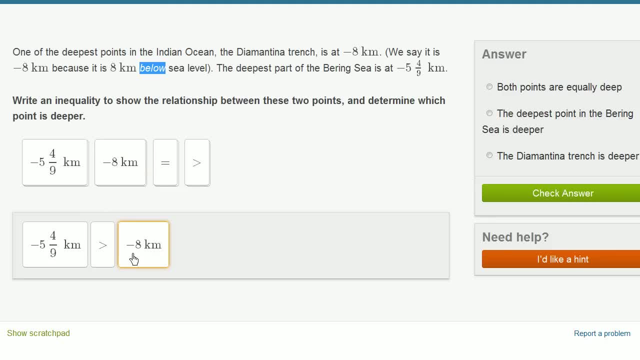 Or negative 5 and 4 1⁄9 kilometers is greater than negative 8 kilometers, And so if we're thinking about which point is deeper, it's going to be the one that's more negative, because that tells us how far below sea level we are. 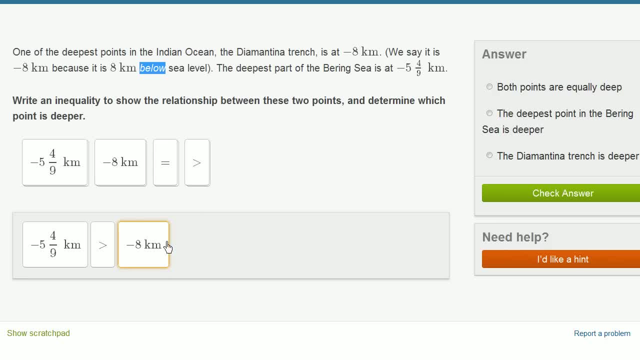 So the negative 8 kilometer point is further below sea level And that is, Let's see Negative 8 kilometers. The Diamantina Trench at negative 8 kilometers is the deeper point And this is fun because in some of these questions 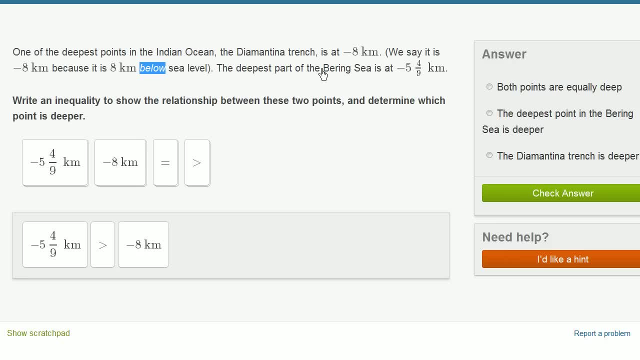 you actually learn things. I always thought that the deep is part of the Bering Sea. Well, anyway, we can talk about that another time. So negative 8 kilometers. So the Diamantina Trench is deeper. Let's do one more.